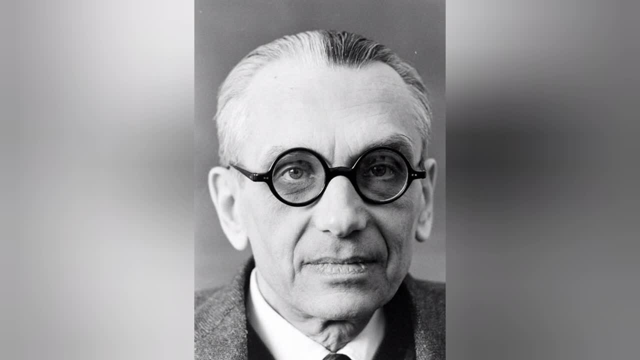 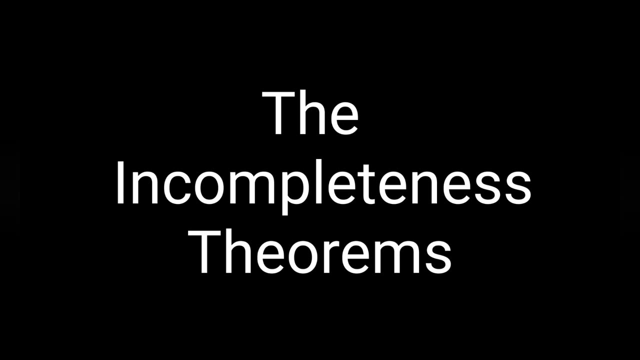 Why would Gödel put so much effort into mathematics if he already proved its futility? Firstly, what is this theorem? Well, in fact, they are the incompleteness theorems, plural. There are two theorems, not just one. The first one is the best known one. 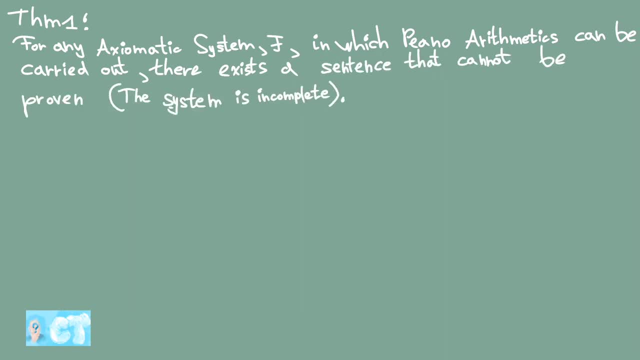 which says that for any consistent axiomatic system F in which piano arithmetic can be carried out, there exists at least one sentence that cannot be proven or disproven, ie the system is not complete, Generally understood, as there will always be. 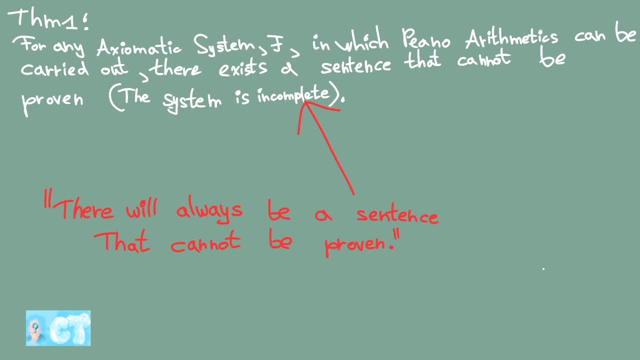 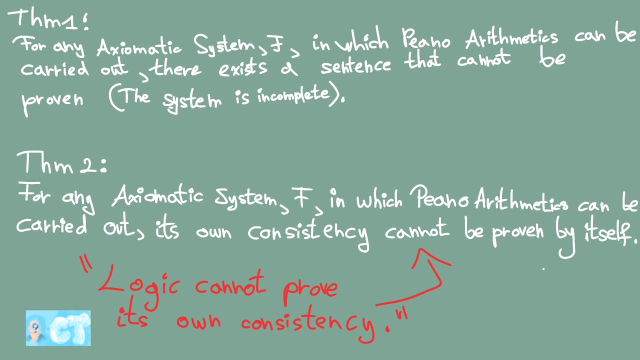 sentences that cannot be proven, But the preconditions are more important than one might think. The lesser known second theorem is that for the same system F, its own consistency cannot be proven by itself, Which can be generally understood, as we cannot prove the consistency of. 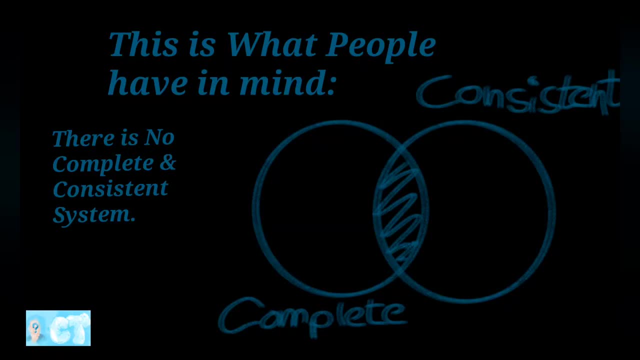 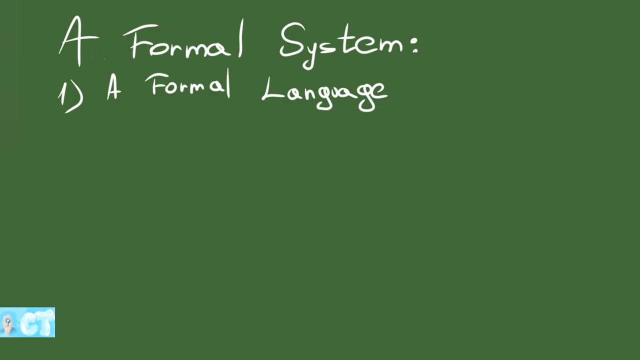 logic, Even though these statements are kinda true. well, it's with an asterix and some caveats. The Gödel's incompleteness theorems are no doubt about it, some of the most misunderstood theorems in mathematics. For starters, what is a formal system? A formal system has these following: 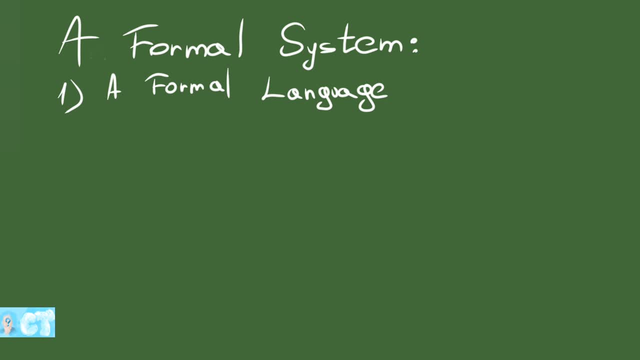 properties. One: it has to have a formal language, which is defined as a structure of two sets of finite symbols, its alphabet, so to speak, and a set of logical connectors and a grammar, a set of rules by which we can decide whether any statement built from them is a well-formed formula. 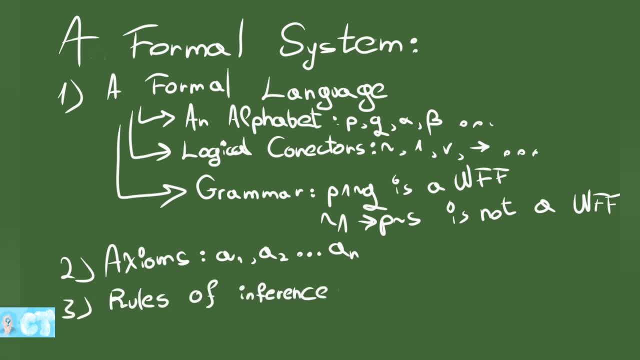 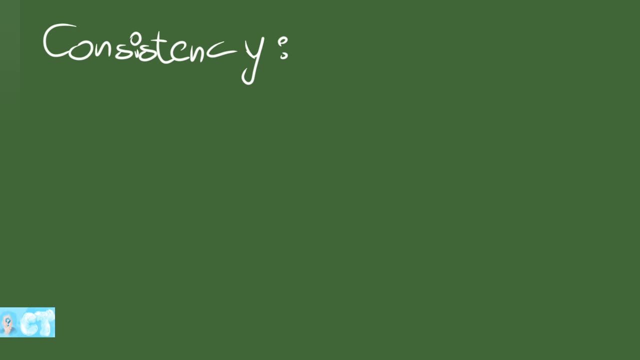 Two, it has some axioms. And three, it has to have some rules with which to infer or prove from the axioms the theorems of this formal system. After that, there are two concepts central to our theorems, namely completeness and consistency. Consistency is an extremely 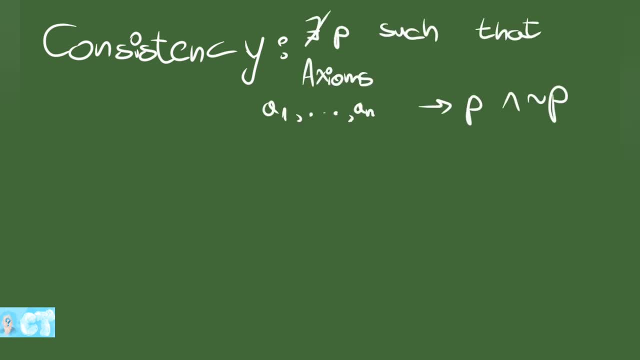 straightforward concept to explain. it only means that in an axiomatic system there is no sentence P such that both P and non-P can be proven. If such a case did happen, we would have an antinomian on our hands and we would have an antinomian on our hands and we would have an 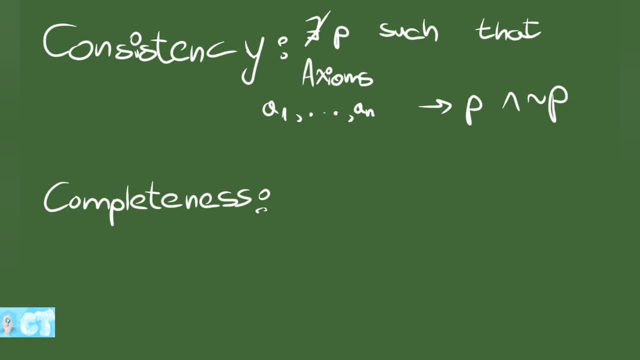 antinomian on our hands, or a paradox. Completeness, on the other hand, means that for any sentence P of said system, there is either a proof for P or for non-P from the axioms of the system. A very interesting case of this is mathematical logic, since, well, it has no. 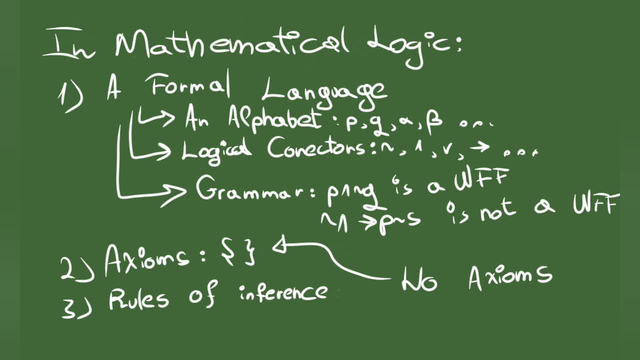 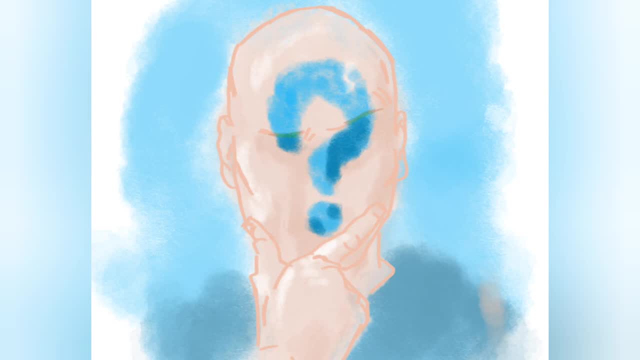 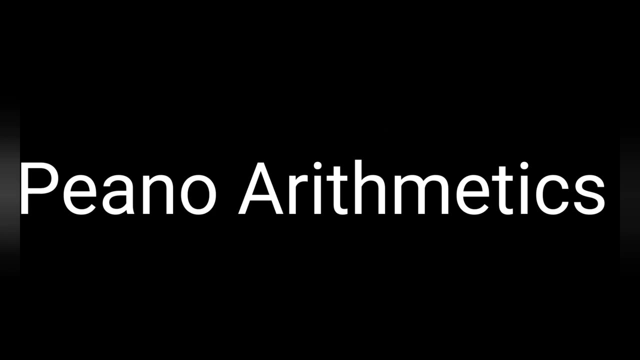 axioms, so to speak. the rules for thought are more descriptions of how to infer, not proper axioms. So, generally speaking, the incompleteness theorems do not apply to it, since it is trivially consistent. Now, what are Peanoarithmetics? The other precondition, generally speaking. 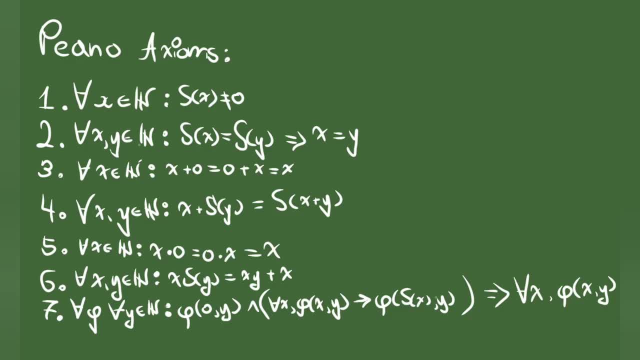 they are a formal system with this following: axioms which are in some way used to build up the natural numbers induction and to define both addition and multiplication, And any axiomatic system that can deduce them or implores them in some way can carry out Peanoarithmetics. 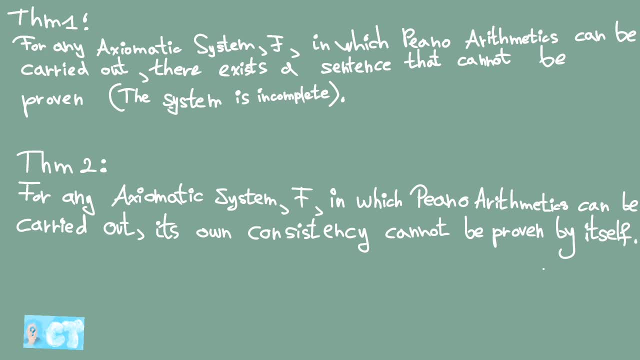 Also as a consequence of the two incompleteness theorems. these formal systems aren't complete and cannot prove their completeness. They are not complete and cannot prove their completeness. They are not complete and cannot prove their own consistency, or they are inconsistent. 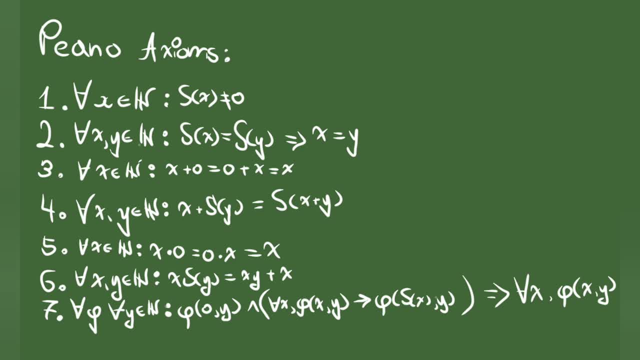 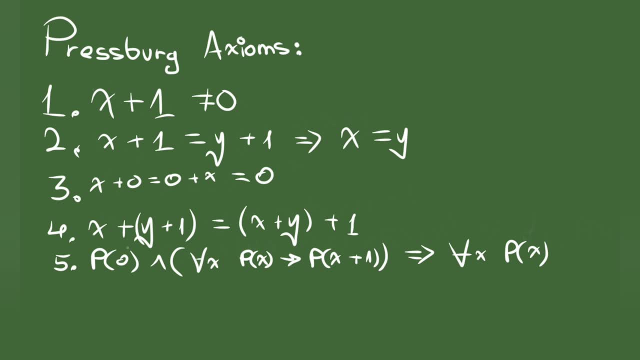 But there definitely are axiomatic systems that cannot carry out such arithmetic operations, such as Pressburg Arithmetics and Skolem Arithmetics. Pressburg Arithmetics is interesting in particular because they do define a way to do addition. 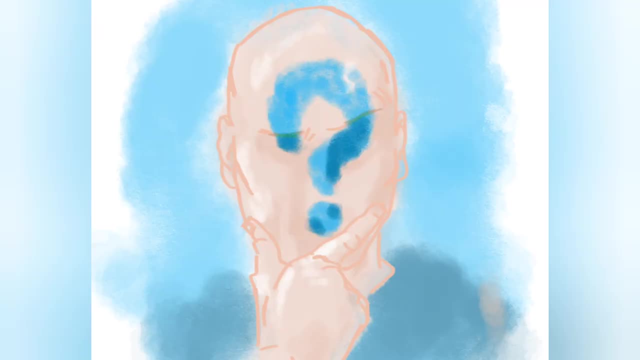 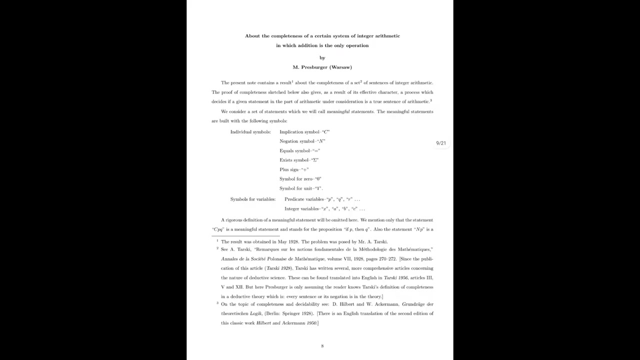 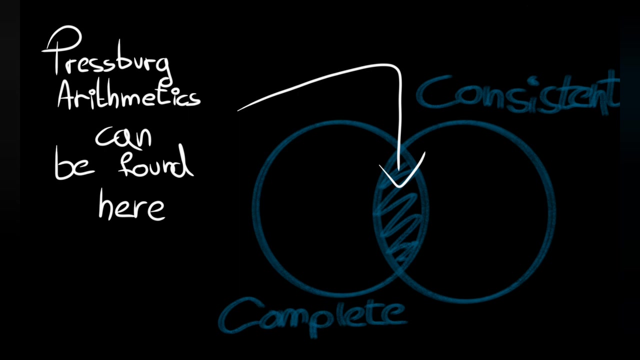 but no way to do multiplication. It is a weaker system, so weak, in fact, that we cannot prove the incompleteness results in it and, in fact, we can prove its own consistency and completeness within itself. Yes, there are such things as complete and consistent axiomatic systems, as surprising as it. 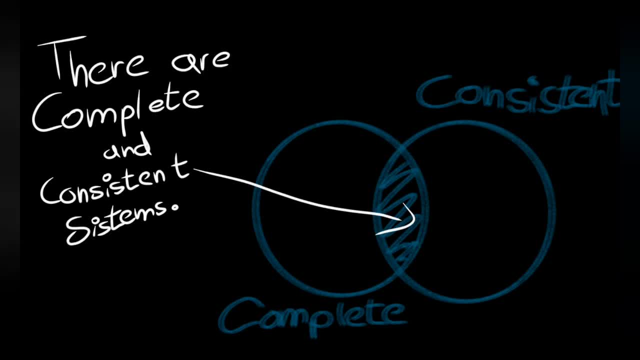 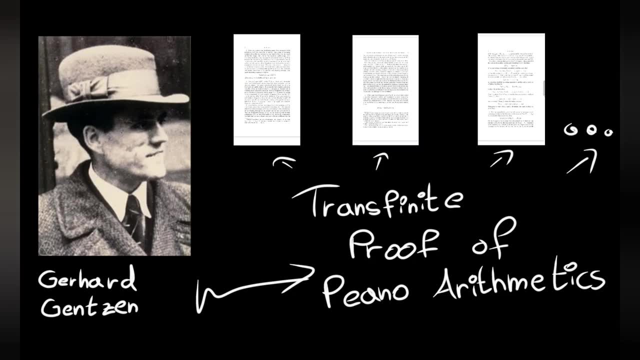 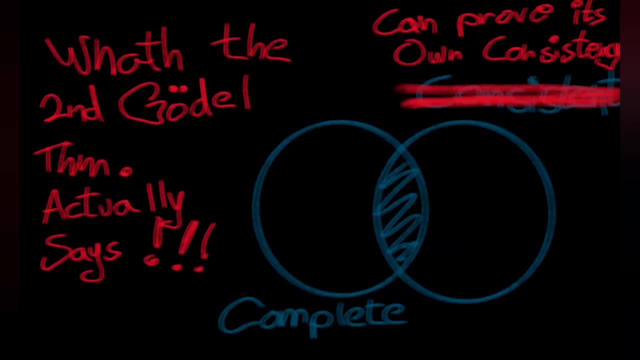 may seem, but this holds for axiomatic systems that cannot carry out Peanoarithmetics, Also the other Skolem Arithmetics. well, in that axiomatic system we can construct a proof for the consistency of Peanoarithmetics. Yes, because this is a different axiomatic system, we can prove the. 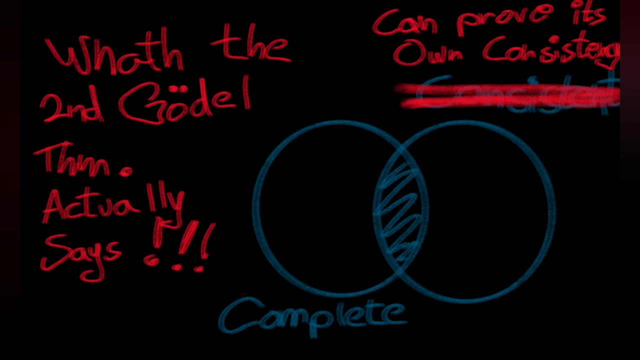 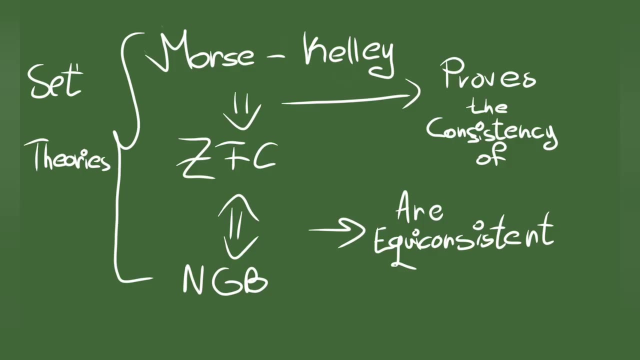 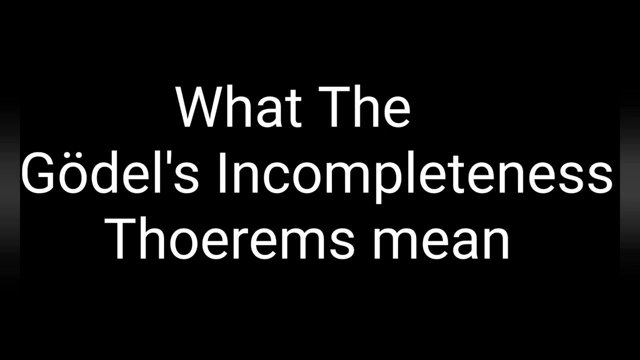 consistency of another. the second Gödel theorem only restricts some systems from proving their own consistency. Actually, a lot of axiomatic theories about set theory can be proven consistent in larger theories And some really weak ones can prove their own consistency. So now that we understand all these, 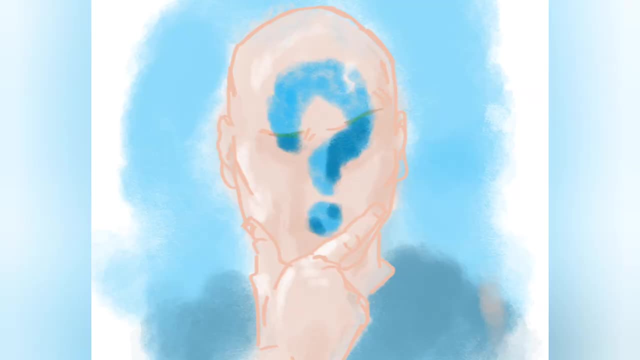 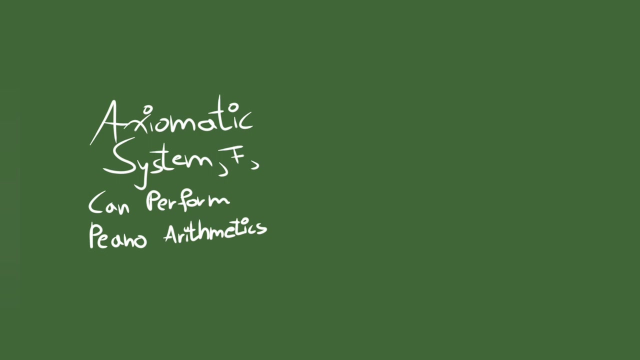 counterexamples to what is commonly believed about incompleteness. we can state what they actually imply Once you form an axiomatic system sufficiently strong to do Peanoarithmetics. that system would be incomplete and you will need a bigger system to prove the original one is.